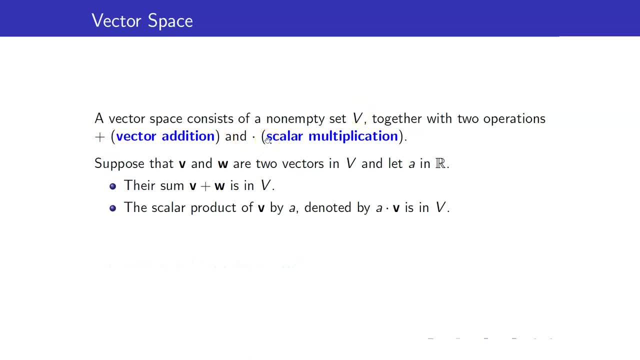 These two operations here must satisfy the two following properties. First, if you get the sum of two vectors, the answer should still be a vector in V. Next, if you have a scalar and you multiply it with a vector V, the answer should still be in V. We say that the set is closed. 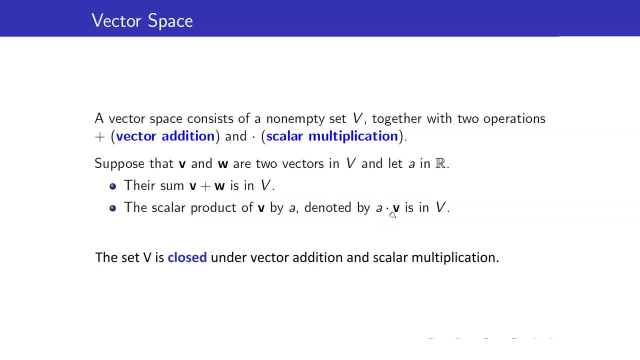 under vector addition and scalar multiplication. Let me just illustrate what this is saying. If this box is your set V and we get any two elements inside the box V, we have V and W. when we get V, we get a set V. When we get V, we get a set V. When we get V, we get a set V. 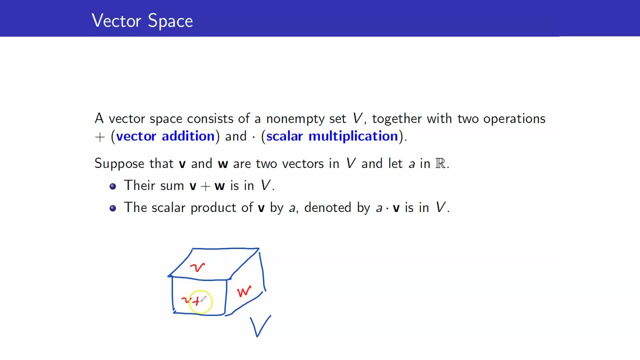 we add them. we should not go outside the box. The answer should still be inside your box. Moreover, if I multiply V with any real number, its scalar multiple should also be in V. Aside from this, a vector space must satisfy the following conditions. Here are 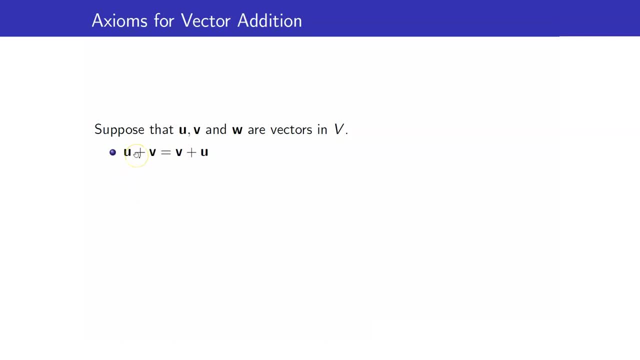 the axioms for vector addition. First, vector addition must be commutative. Second, it must be associative And there must be a zero vector. The zero vector is just like your real number zero. When you add a zero vector with any vector, you should get the vector itself. 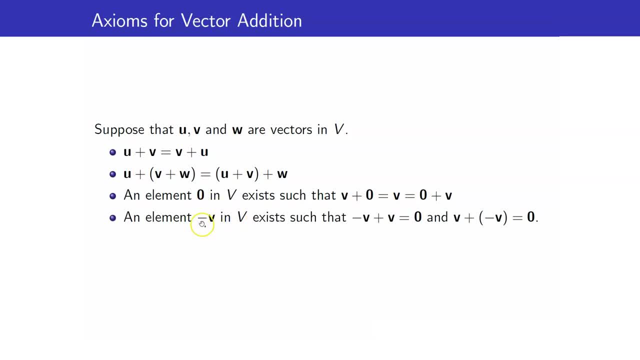 Moreover, every vector should have an additive inverse. When you add an additive inverse of an element with a vector, you should get the vector itself. With that element, we should be able to get the zero vector. Here are the axioms that must. 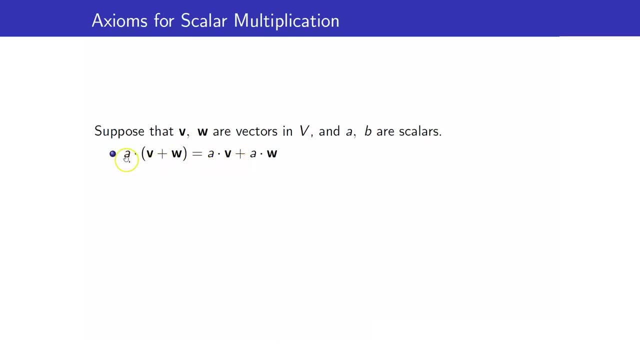 be satisfied for scalar multiplication. First, it should be distributive. When we multiply a scalar with the sum of two vectors, it's the same as getting the scalar multiple of each vectors and adding those. Second, we also have some sort of distributive property. 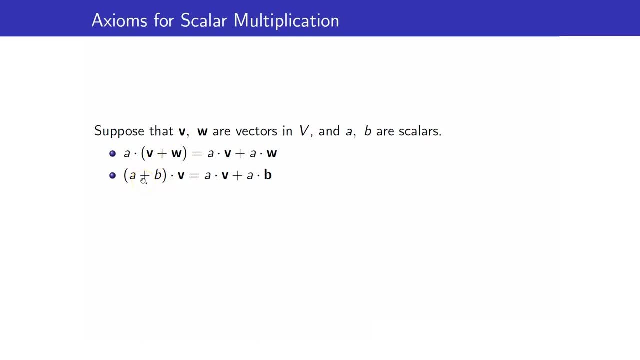 here. But take note that the addition here is the sum of the two vectors. So if we add a scalar with the sum of two vectors, we should get the vector itself. This addition over here is your vector addition in V. Maybe I should write this one: V, Whereas the addition 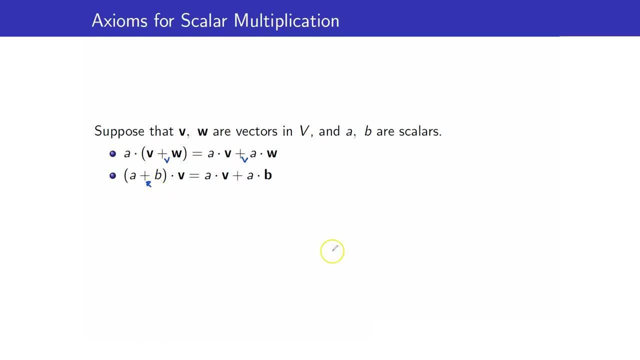 here is your addition in real numbers. Let me just write R. Whereas here, what kind of addition is this? This is the vector addition in V. Next, scalar multiplication should be associative as well. Again, this is the scalar multiplication defined in V, whereas here this product AB, here this is multiplication in the 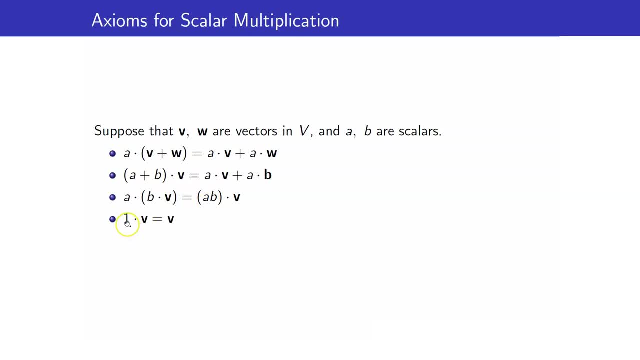 set of real numbers. When we multiply the real number 1 with any vector V, we should get the vector itself. How do we check if a set with operations is a vector space? First we have to identify the set V of objects that will become vectors. Once we have identified that, it's also 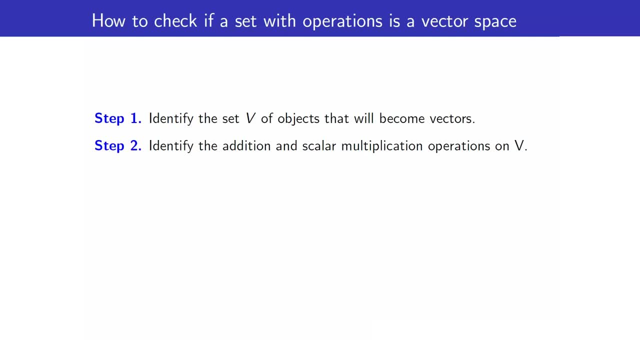 important that we identify the addition and scalar multiplication operations in V. Now the third step. here is the most important part. You have to check this too- that the set V is closed under addition and multiplication When we add two vectors it should still be in V When you get. 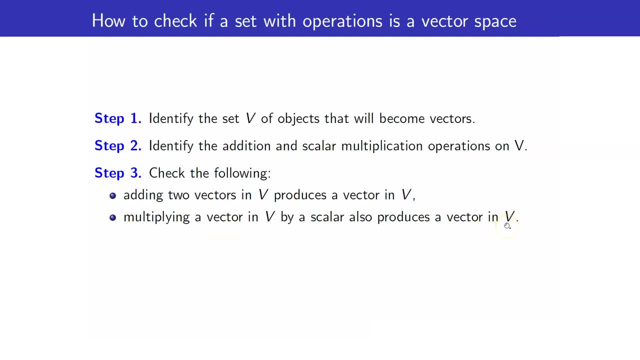 a scalar multiple of any vector, it should still be inside V. Once you check these two properties, you may now proceed in checking the other properties. Why is it important that we have to check this first? Take note that the other properties would not make sense if these two are. 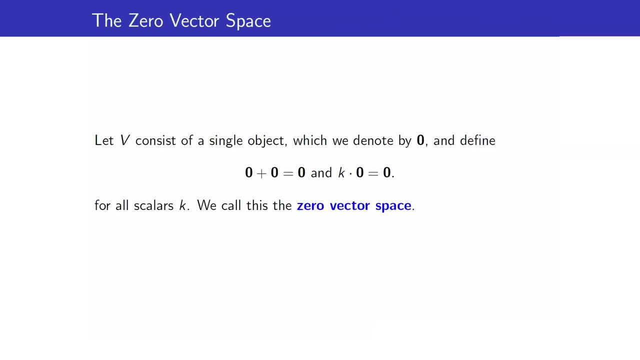 not even true in the first place. Let us have our first example of our vector space. Suppose that V consists of a single object only, which we denote by the 0. This is our 0 vector, and we define this: 0 plus 0 equals 0, and any number times 0,. 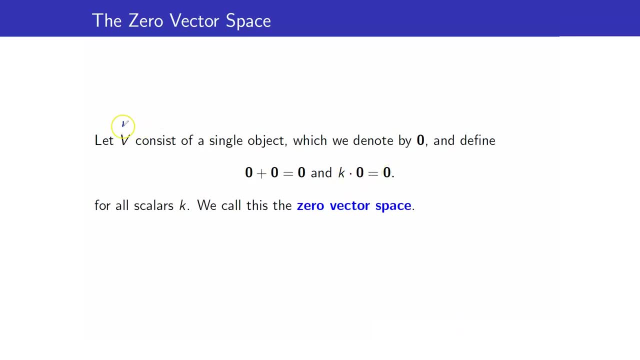 is equal to 0.. We have our step 1 already. We know what our V is. It just consists of a single object. We know the operations addition and scalar multiplication. In step 3, we just have to check your closure property. But of course when you add 0 with itself, the answer is still inside the 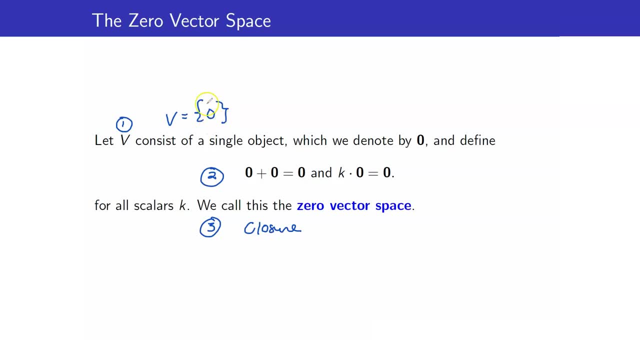 set. When you multiply 0 with any scalar, it should still be in V. So we have to check this first. Step 4, we have to check the other properties. But the other properties it's very trivial because it's just 0 anyway, I will leave it up to you. We call this the 0 vector space, or. 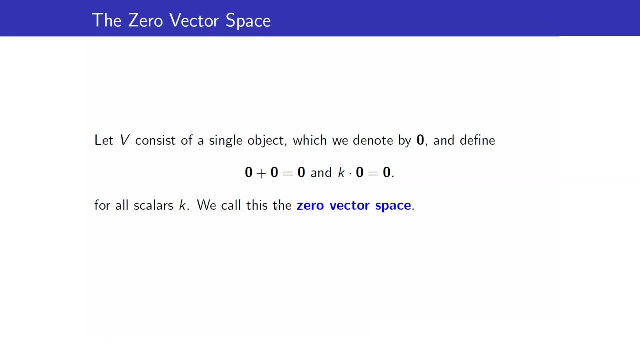 the trivial vector space, because it only consists of a single object. Next, let us consider the set of all integers with standard operations. We have to check the other properties and we have to check the set of all integers. Is this a vector space? Step 1, we have to identify our V. Our V is: 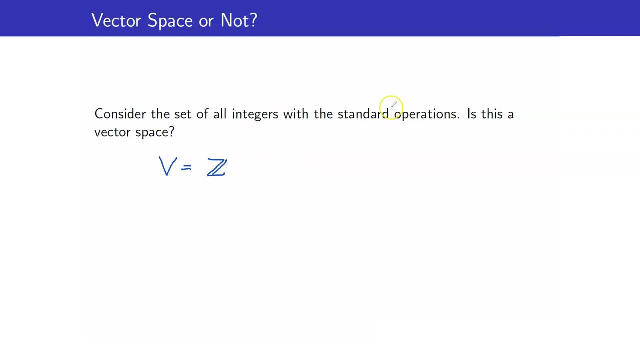 the set of all integers. What do we mean by standard operations? So what is now vector addition here? This vector addition is the usual addition of integers. Take note here that U and V are vectors, So therefore they must be integers. Next, if I multiply: 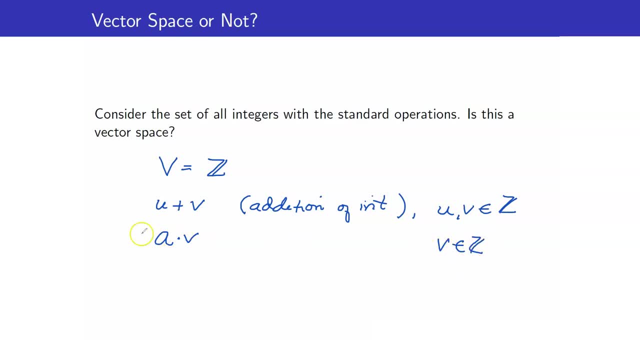 a vector V. take note: V is an integer. What about our A? A is a scalar, So therefore A is a real number, A dot V is just multiplication. All right, So we're done with step 1.. We're done with step 2.. 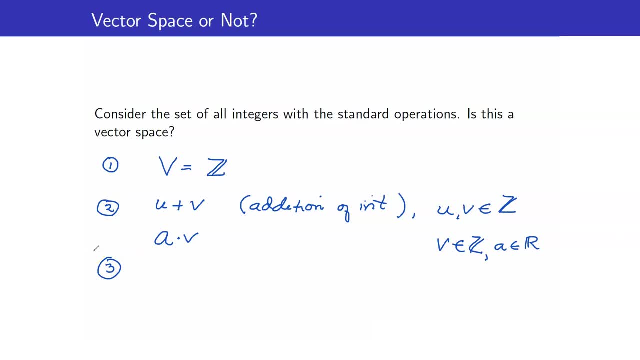 Step 3, let's check for the closure property. Is this closed under addition: When we add 2 integers, do we get another integer? Yes. Is it closed under scalar multiplication: When we multiply a real number with an integer, do we get another integer? No. For example, my A is 1 half If I multiply. 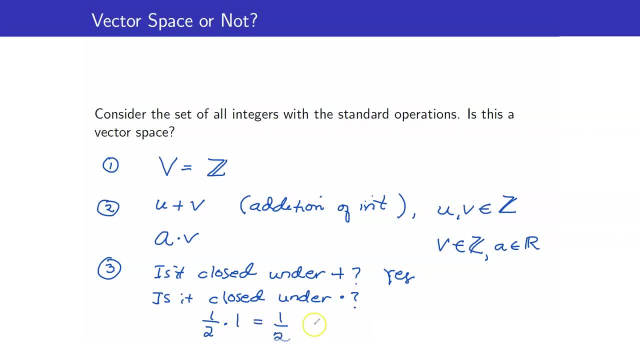 that with an integer 1, the answer is 1 half, which is not in V. Your 1 half here is your scalar, Your 1 over here is your vector. So we have a scalar times a vector in V. The answer is not another. 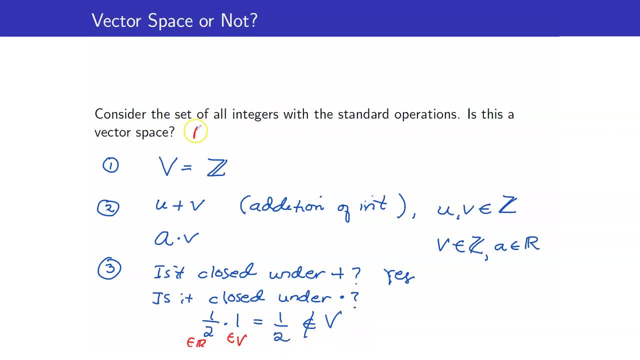 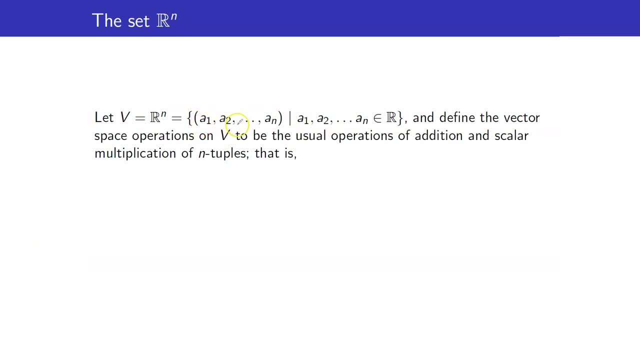 vector in V. So therefore the answer here is no. Next, let us consider the set of n-tuples. We have A1, A2 up to An. These are just real numbers, or we say that V is a set of n-tuples. 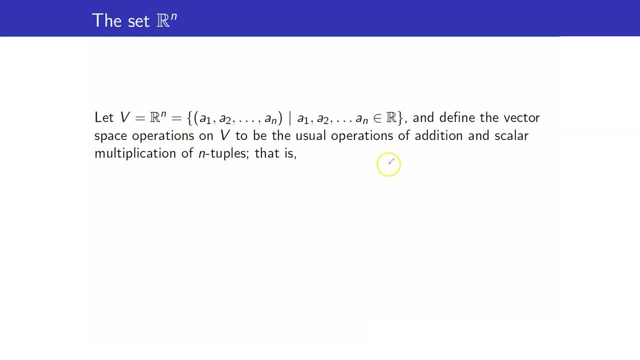 And we define the vector space operation to be the usual operations of addition and scalar multiplication. These are our two vectors, u plus v. When we add two vectors, two n-tuples, here we get this n-tuple. This is a scalar, This is a real number. 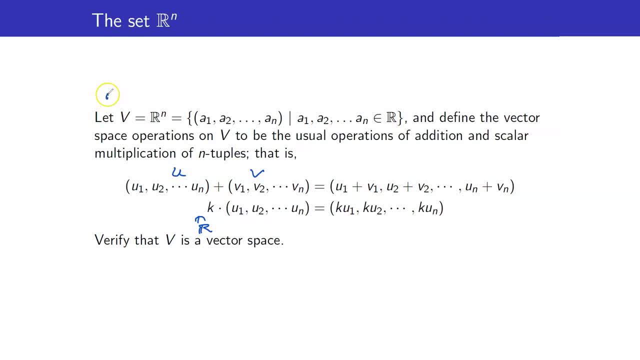 Verify that v is a vector space. Step 1, we already identified our set v. It consists of n-tuples. Step 2, we have identified already our operations, our vector addition and our scalar multiplication. Step 3 is the closure property. 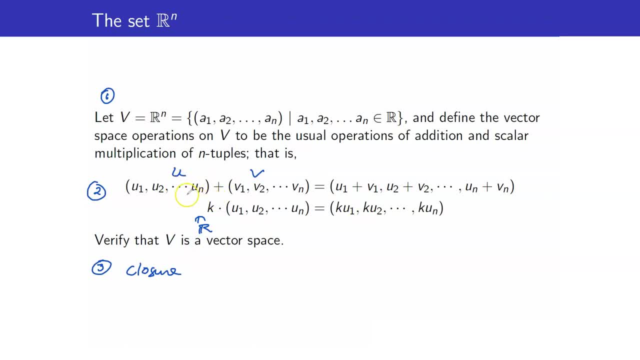 Is it closed under addition? Look at this one. If I add two n-tuples, the answer is still another n-tuple. Therefore, it is again inside the set v. If I have a scalar and I multiply it with an n-tuple, the answer is again another n-tuple. 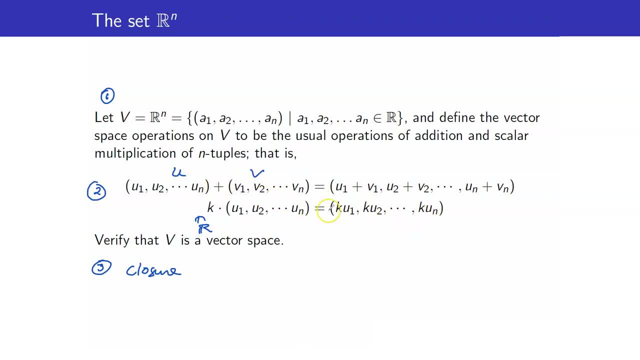 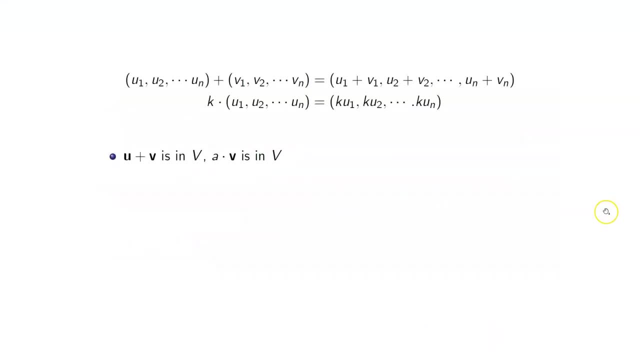 Therefore it is closed. under vector addition and scalar multiplication. Let us check the other properties. We've already finished this. Is it commutative? This is my u plus v. If I add v plus u first, will I get the same number? 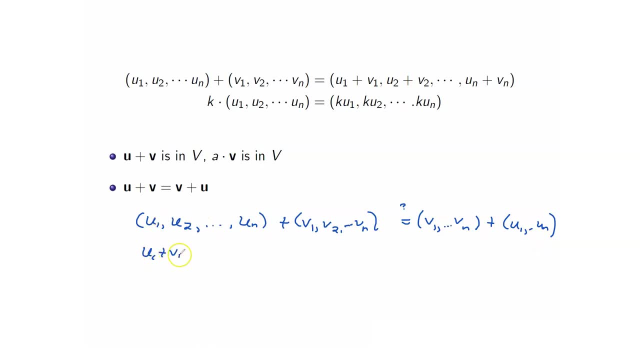 This is equal to u1 plus v1,, u2 plus v2, and so on. However, this addition over here is addition of real numbers, correct, And addition of real numbers is commutative. I can switch this as v1 plus u1, v2 plus u2, and so on. 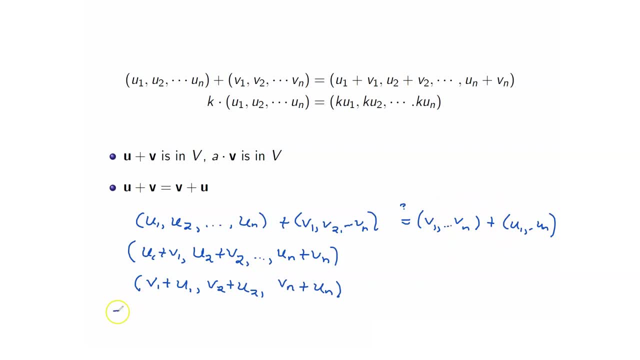 And take this as v1 plus v2.. And take this as v1 plus v2, and so on. And take note that that is exactly this one over here. So therefore u plus v is the same as v plus u. I will leave it up to you to check that it is associative as well. 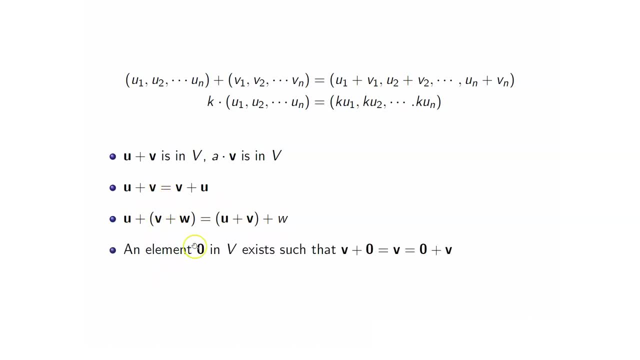 It's almost the same as this one. Next, we have to identify if there is a 0.. What is the 0 element in our vector, space v? Our 0 vector is: what do you think? This is the n-tuple consisting of 0s. 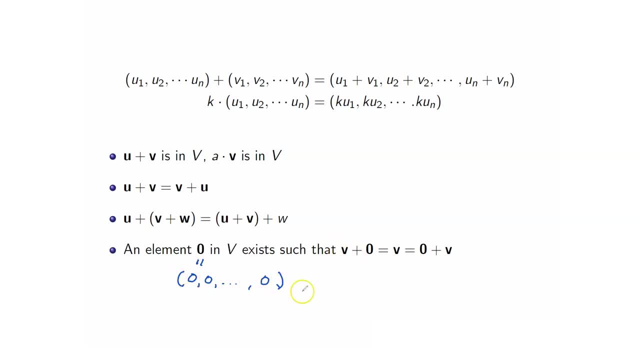 Because if you have an n-tuple, when you add it with this n-tuple over here, you get that same n-tuple. Next we have to check if the additive inverse of any vector exists. If my v is v1 up to vn. 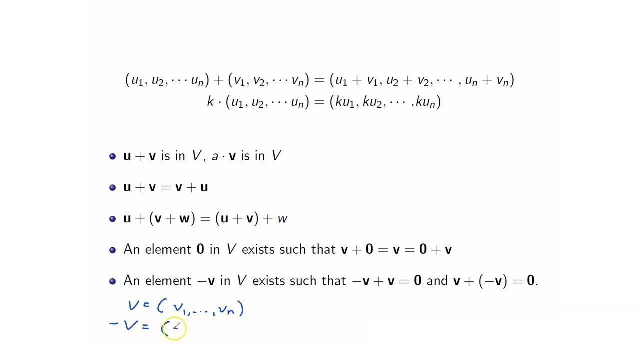 What is my additive inverse? It would be negative v1 up to negative vn. Correct, When you add this two, you would get the 0 vector, which in this case is the n-tuple consisting of all 0s. I will leave it up to you to check this for other properties. 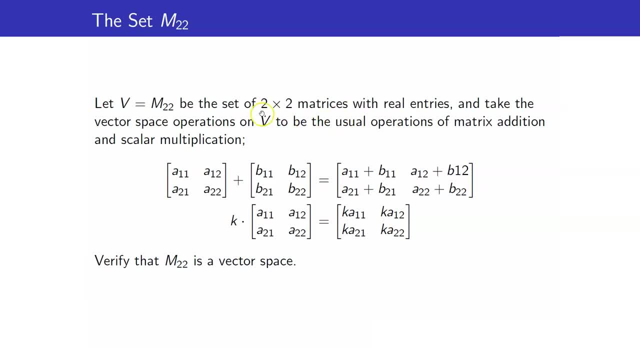 Next, let us consider the set of all 2x2s. Next, let us consider the set of all 2x2s. Let us consider the set of all 2x2s with real entries and take the vector space operations on v to be this: 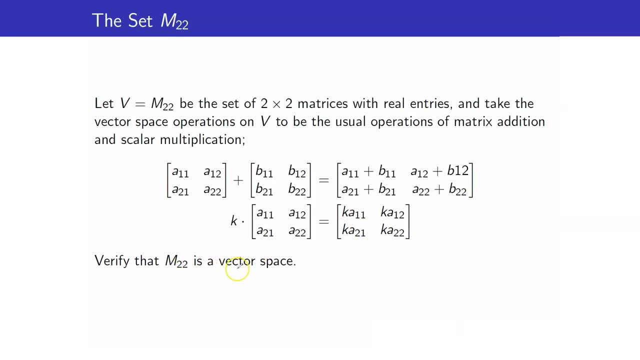 Let us verify that this is a vector space. Our set v is this set set of 2x2 matrices. Next, these are our operations: We're adding two 2x2 matrices and this one k is our real number here. 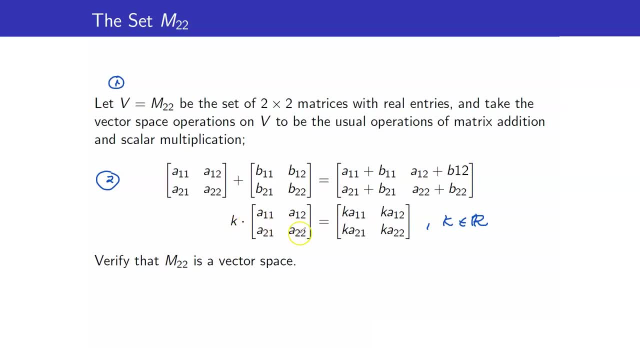 That's just the usual And scalar multiplication of matrices. Let us verify that this is a vector space. Our very important step is step 3, identify if it is closed under addition. From here, if you add two 2x2 matrices, the answer is again another 2x2 matrix. 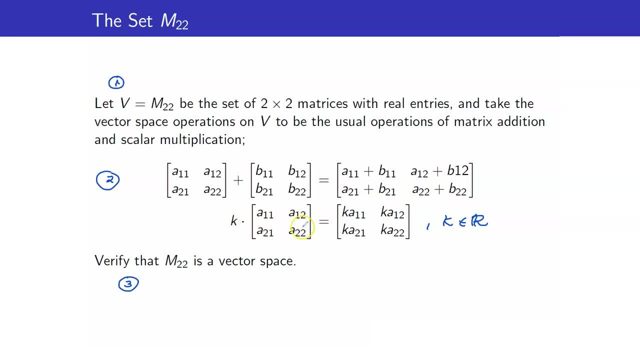 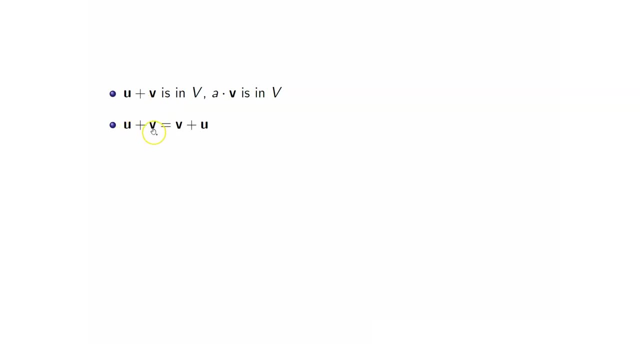 If I have a scalar multiplied to a 2x2 matrix, the answer is again another 2x2 matrix. So therefore, yes, it is closed. under addition, Addition and scalar multiplication, We're done with this- Is addition of matrix commutative. 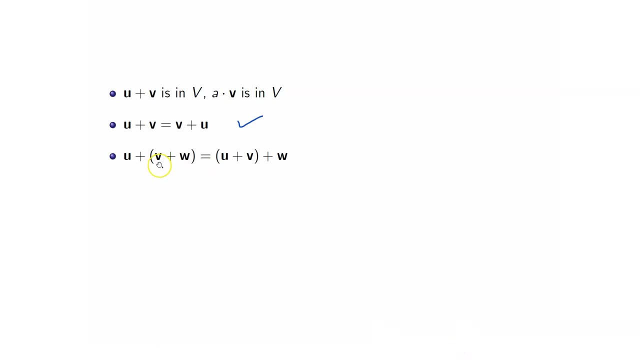 Yes, Is matrix addition associative? Yes, We've seen this in our previous lectures. What would be our zero vector here? Our zero vector would be the 2x2 matrix, wherein all entries are 0.. Next, if we're given a vector, 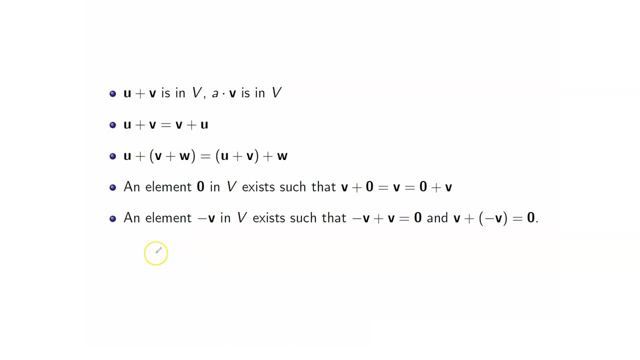 remember that a vector here would just be a 2x2 matrix. Let's say we have a, b, c, d. What would be your negative v here? Of course it's just the usual negative of a matrix: Negative a, negative b, negative c, negative d. 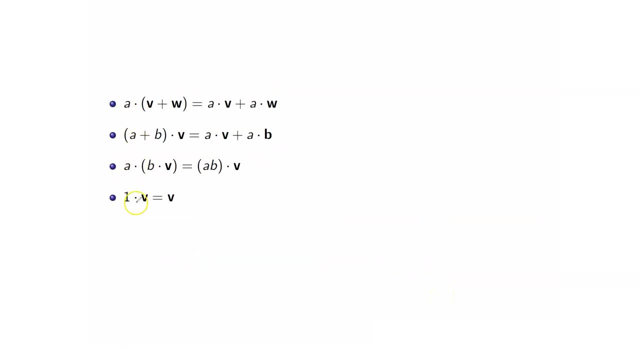 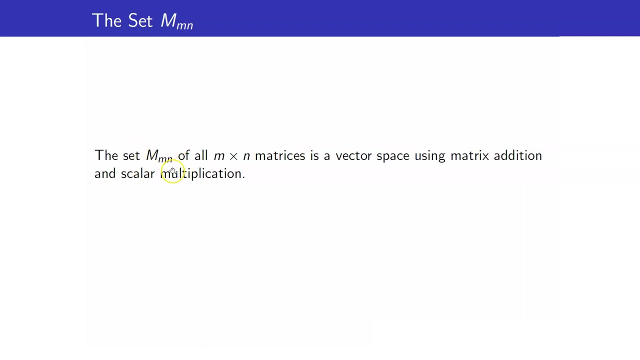 And then all of these properties. we have seen from our previous lectures that this will still be true in the set of matrices. Remember here again that v and w are 2x2 matrices. We can actually generalize what we did in the previous slides for the set M, M, N. 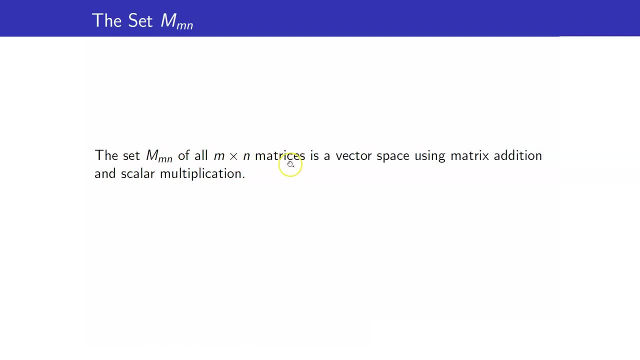 What is this? This is just a set of all M by N matrices. We don't have to confine ourselves to 2x2 matrices. Whatever we did in the previous slides is still true in general for any matrix of size. So if we collect all the matrices of size M by N, 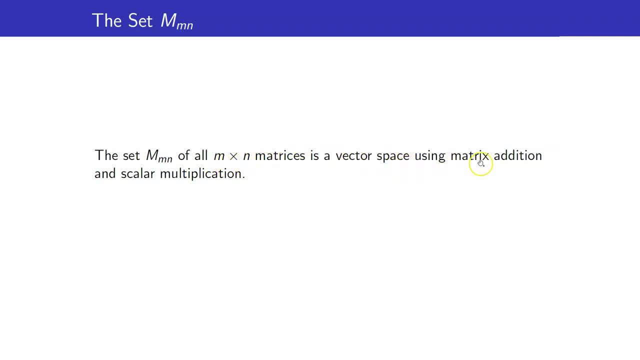 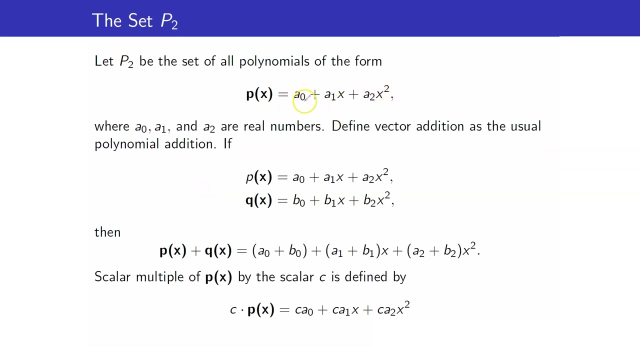 that would be a vector space wherein vector addition is matrix addition, and the usual scalar multiplication of matrices will be your scalar multiplication. Next, let us consider the set of all polynomials of this form. Take note here that a0,, a1, and a2 are just real numbers. 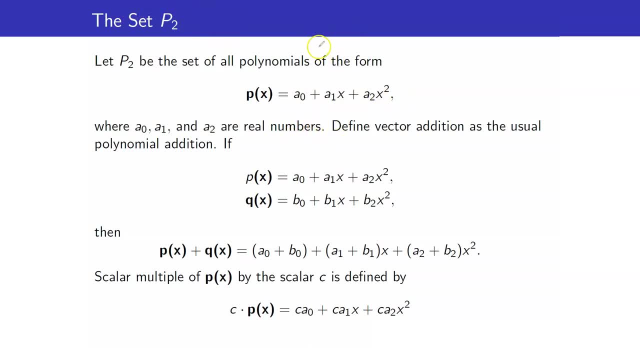 What is this saying? p2 is just a set of all polynomials of degrees. p2 is just a set of all polynomials of degrees. p2 is just a set of all polynomials of degrees less than or equal to 2.. 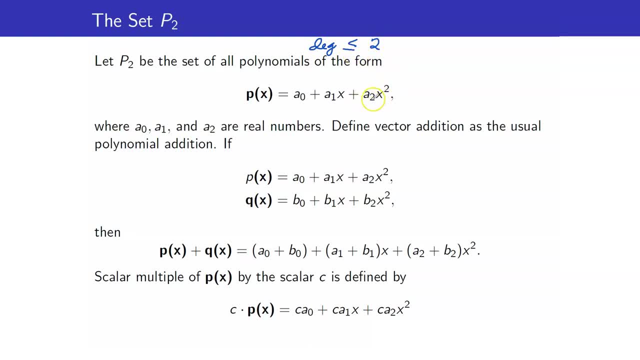 Why is it less than or equal to 2?? Because if a2 is 0,, then this would just be of degree 1, correct. You can also have a2 and a1 to be 0. And if that is the case, the polynomial would just be a constant. 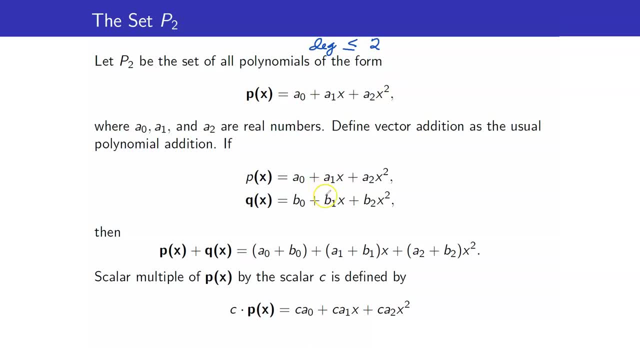 We define our vector addition to be the usual polynomial addition. I wrote this in bold to indicate that they are the vectors, And when it's not bold, that means that it will be a scalar, just like in this case. So if we add two vectors, so in this case our vectors are just two polynomials. 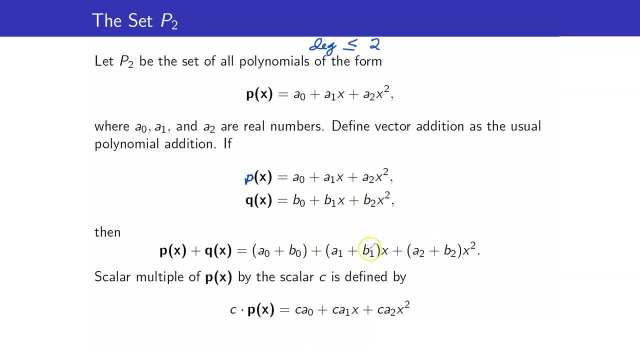 How do we add them? It's just the usual addition of polynomial, And a scalar multiple of p of x is just the usual multiplication. We multiply c with the polynomial. We're done with step 1.. This would be step 2.. 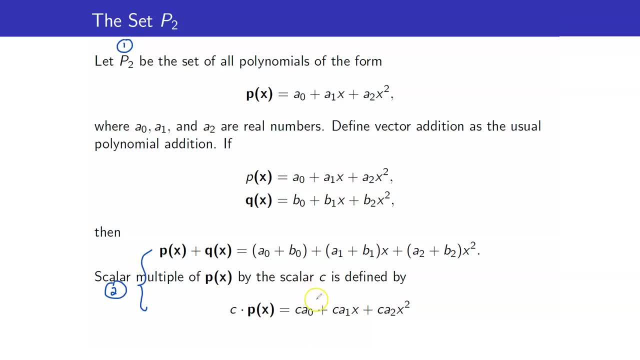 Step 3.. Is it closed? If I add two polynomials, do I get another polynomial? Yes, If I have a scalar and I multiply it with another polynomial, is it another polynomial? Yes, as well. So therefore it is closed under vector addition and scalar multiplication. 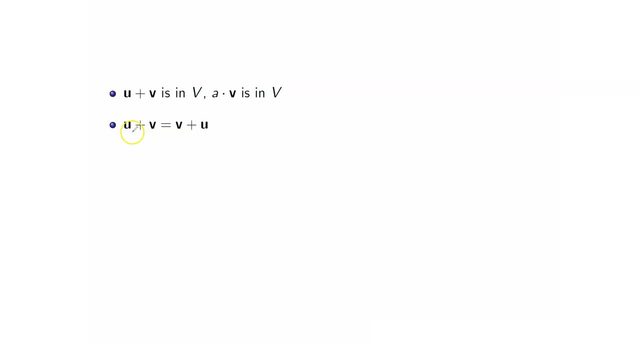 Next, is it commutative? Is it commutative? Is polynomial addition commutative? Yes, Is polynomial addition associative? That's yes as well. What is our zero vector? Our zero vector would be the zero polynomial. But the zero polynomial is just the real number, zero, correct? 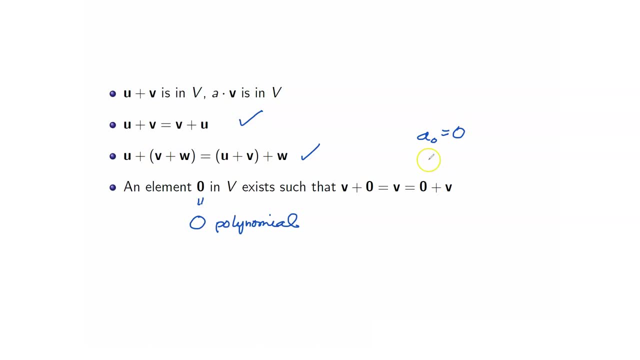 Meaning to say your a0 is equal to zero, a1 is equal to zero and a2 is equal to zero. Next we have to identify our additives. Additive inverse, Let's say v is just a polynomial a0 plus a1x. 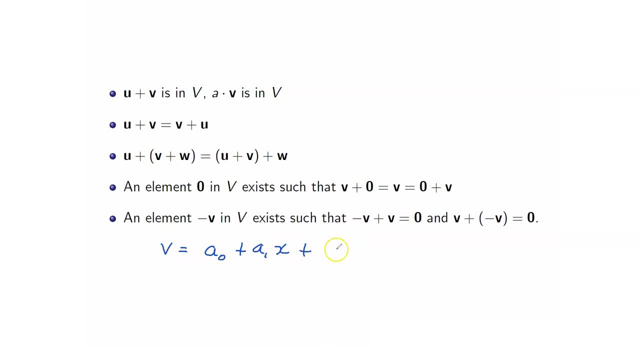 Take note that here you have to get an arbitrary vector. An arbitrary vector is just a polynomial. in this case, What would be its additive inverse? It would be negative a0 minus a1x minus a2x, squared correct. Next, is it distributive. 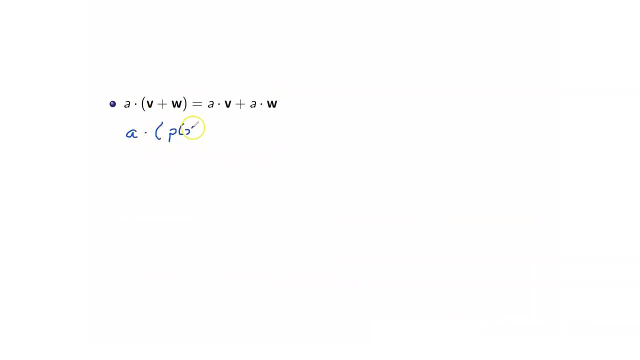 Yes, We have a times a polynomial plus another polynomial. This is the same as a times p of x plus a q of x, right? So this one here is satisfied as well. Again, I will leave the rest as exercises. Hence we've seen that the set P2, together with the two operations defined above, forms a vector space. 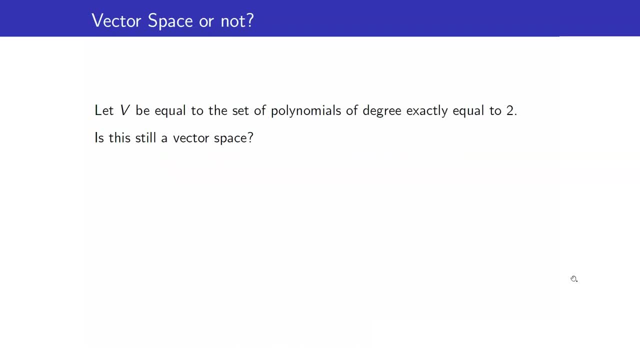 What is the derivative? What if, in this case, we just restrict ourselves to set of polynomials of degree exactly equal to 2?? Meaning to say, our v is of this form: a0 plus a1x plus a2x, squared, where a0,, a1, and a2 are real numbers. 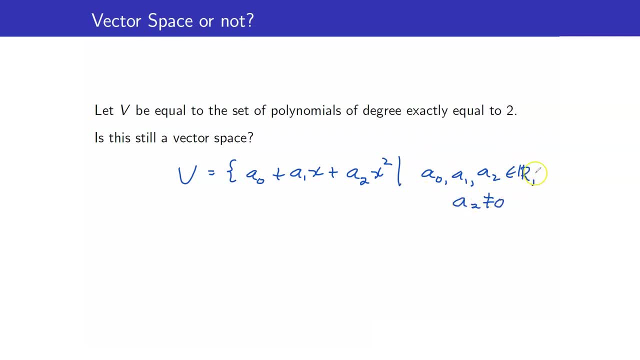 However, we have the added condition that a2 is not equal to zero, to make sure that the degree is exactly equal to 2.. What if, in this case, we just restrict ourselves to set of polynomials of degree exactly equal to 2?? 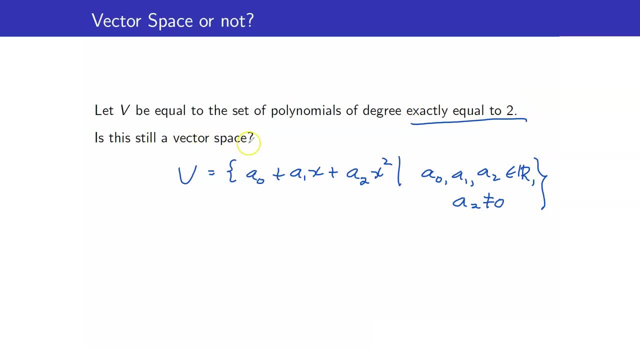 Will this be a vector space? And of course the operations here would be the usual polynomial addition and scalar multiplication. Is this still a vector space? Take note that the answer is no. Note that it is possible that when we get two polynomials of degree exactly equal to 2, the sum may not be of degree 2.. 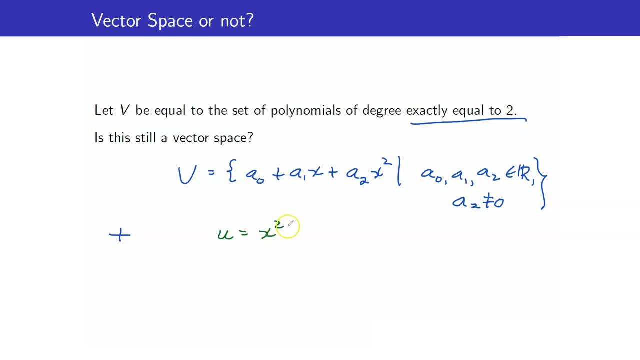 Why is that So? for example, my u is x squared plus x And my v is negative x squared plus 1.. If that is the case, your u plus v would be equal to x plus 1. And that is not in v. 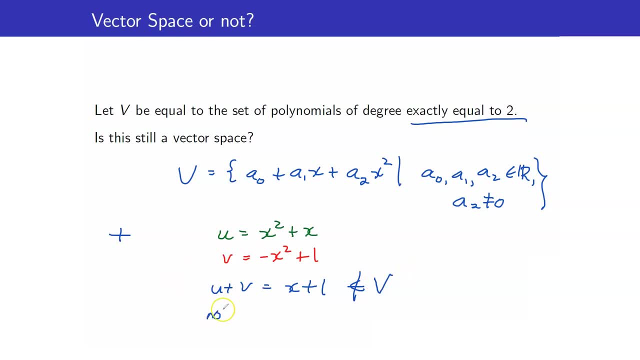 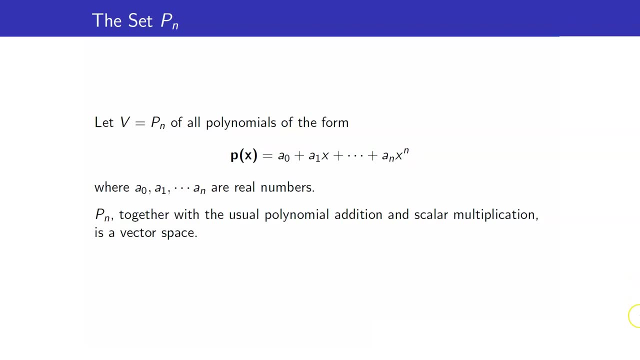 So therefore it is not closed under addition. So therefore the answer here is no. We can actually generalize what we did in the set T2.. If we generalize it to the set Tn, this would be the polynomials of degree- take note- less than or equal to n. 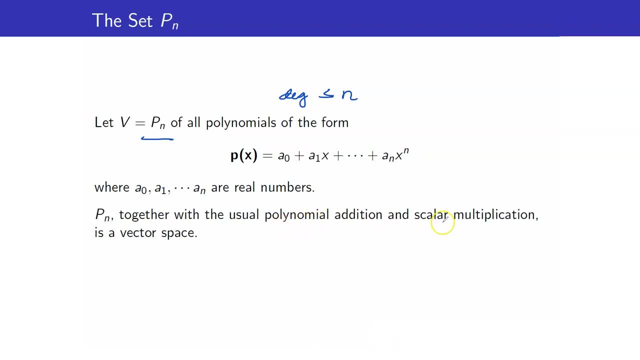 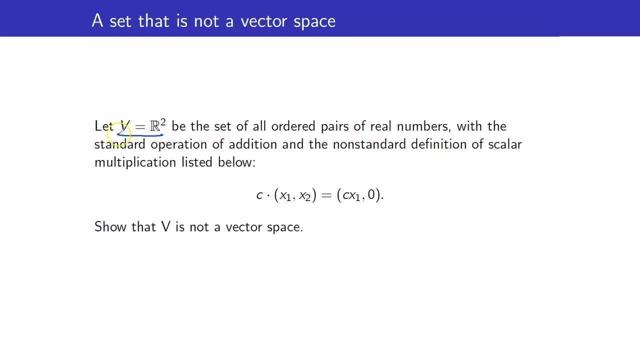 This will form a vector space with the usual polynomial addition and scalar multiplication. Let us look at another example of a vector space. Our set v: here is the set of ordered pairs. Next, step 2, we have to define our addition. Vector addition here is, it says, standard operation of addition. 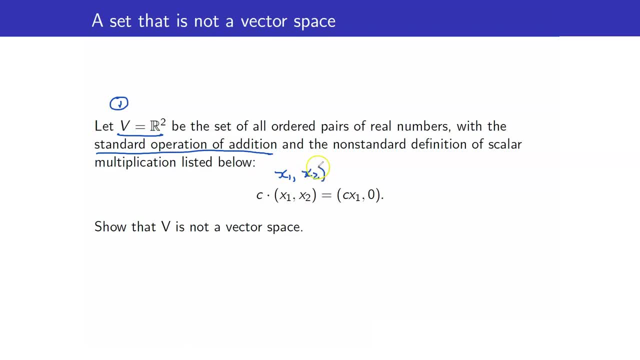 It means that we have x1, x2 added with another ordered pair. It is standard operation of addition of ordered pairs x1 plus x2, y1 plus y2.. But take note that scalar multiplication here is defined to be this one. 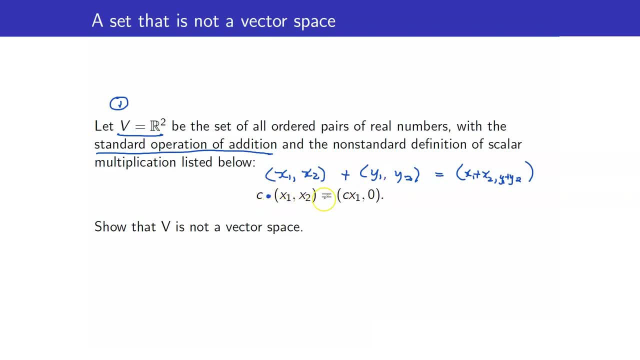 To multiply a scalar with an ordered pair. what you do is you multiply the scalar with the first number, but the second entry will always be equal to 0. This would be our operations. That is step 2.. Step 3, we have to check if it is closed. 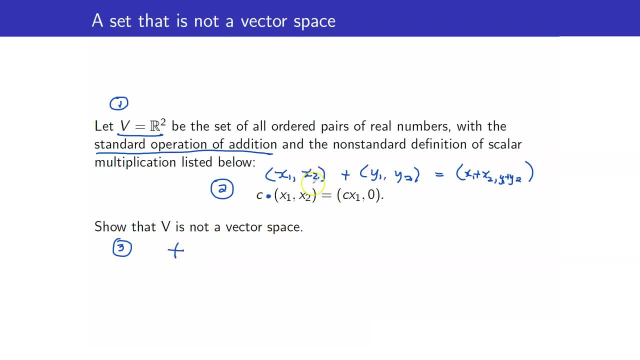 First, is it closed? under addition, We have two ordered pairs. Is the sum again another ordered pair? Yes, If we have a scalar times an ordered pair, the answer is again another ordered pair. So those are satisfied. Let us check for the other properties. 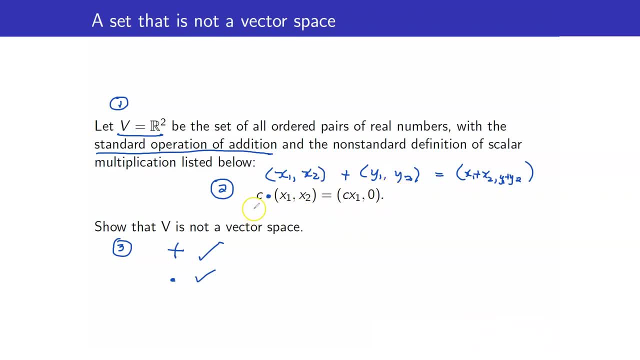 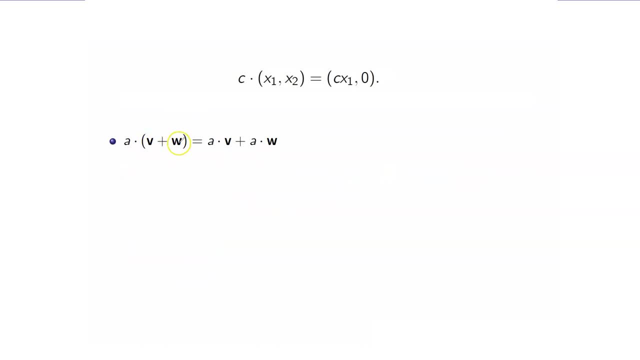 I will first check for the axioms concerning scalar multiplication, because this is a bit different. So first, suppose, let us get two vectors here. This is my vector v, this is my vector w. Is this the same as this one? Let us look at the left hand side first. 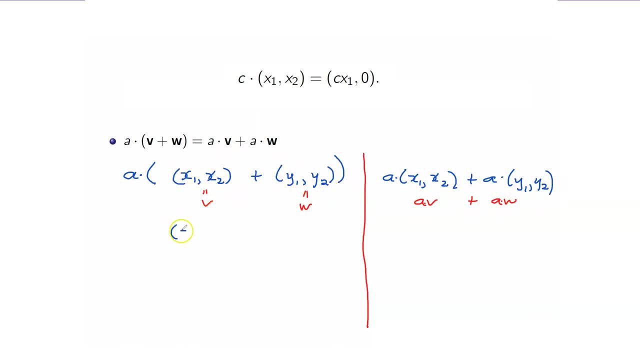 v plus w is x1 plus y1, x2 plus y2.. Then I multiply that with a. But according to our definition I will multiply a to the first coordinate, but the second entry will always be equal to 0.. Let us look at this one, the right hand side. 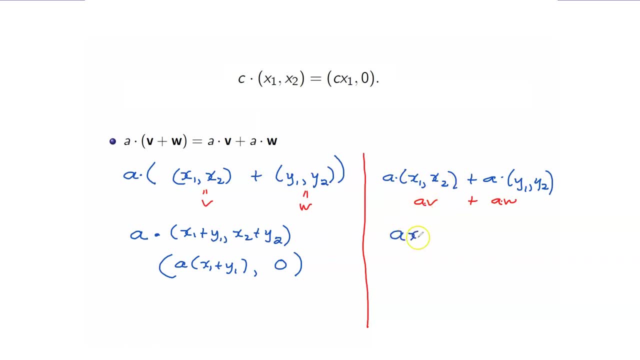 a times v, a times x1,. x2 is ax1, and then 0.. When we multiply a scalar with an ordered pair, the second entry will always be equal to 0, plus a. this is y1, and then 0. 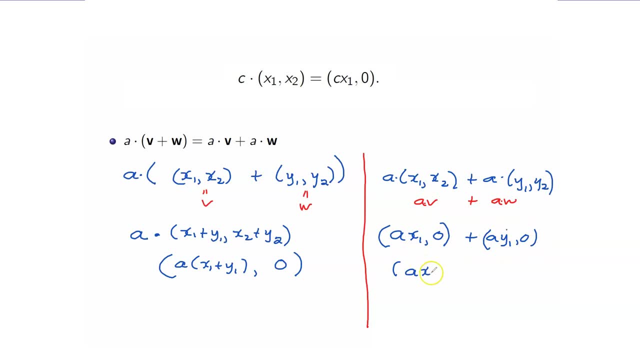 When we add these two, this is ax1 plus ay1, then 0. They are the same. So this is true. Next, let us verify this one. I will use red for my scalar. I will multiply it with my vector. 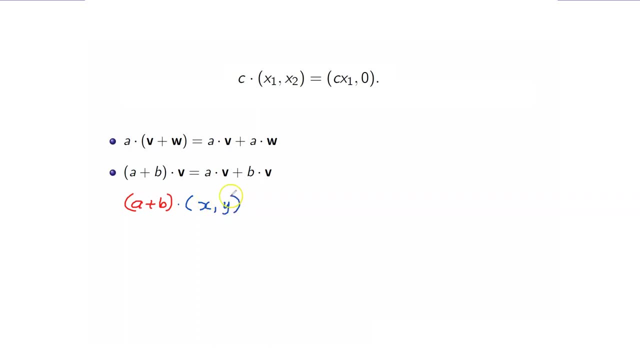 I will use blue for that. We want to check if a plus b times an ordered pair is equal to this. Let us look at the left hand side. We have a scalar times an ordered pair. What happens is you just multiply the scalar with your first entry here. 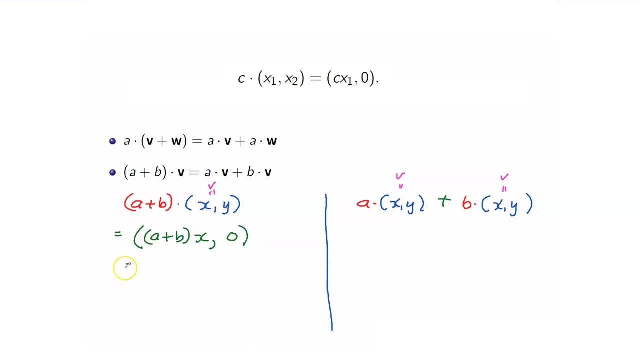 and the second pair would be 0.. This is ax plus b Plus bx 0.. Let us look at the right hand side. here a times xy is ax 0.. Plus b times xy bx. The second entry will be 0.. 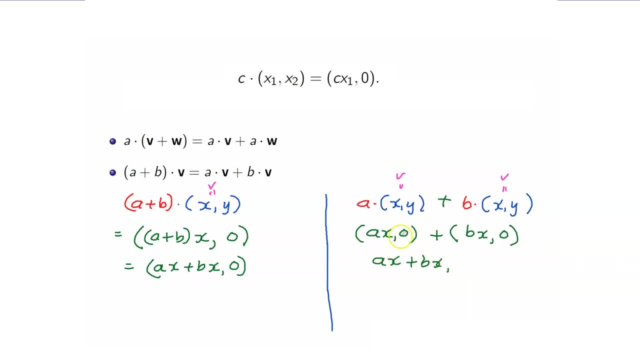 This is ax plus bx. 0 plus 0 is 0. Therefore, this is again true. I will leave for you to verify if this is true. I will just check. if this is true, 1.v is it equal to v? 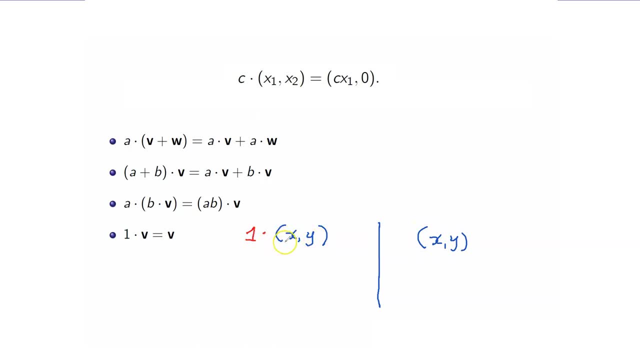 The left hand side is 1 times an ordered pair. This is equal to 1 times x, and the second element is 0, which is the same as x0.. This is the left hand side, Whereas the right hand side, v, is xy. 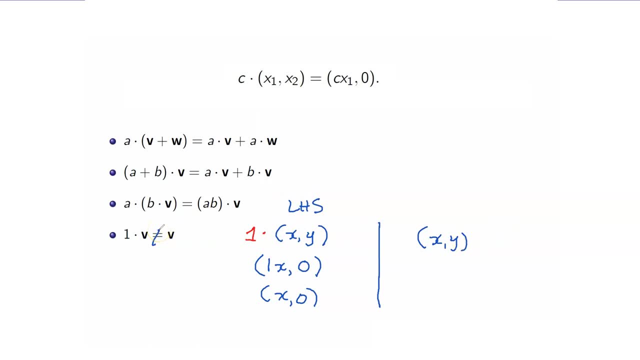 Therefore, this is the property that was not satisfied. Hence, this is not a vector space. I could have shown you earlier that this is not satisfied, but the reason why I did this theory is so that you would be trained on how to verify properties. 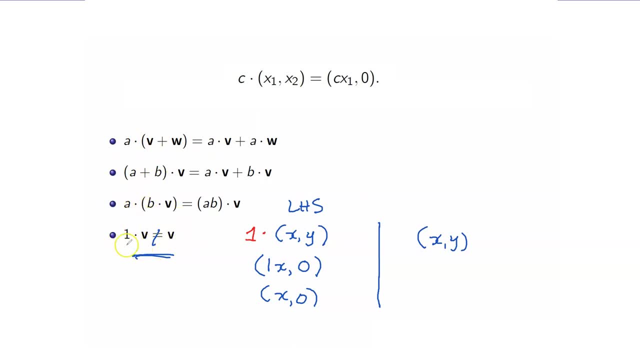 But, of course, if you were able to realize immediately that this will not be satisfied, because of the fact that we have c times xy is equal to cx0, it automatically kills the second element- You should have an idea by then that this one would not be satisfied. 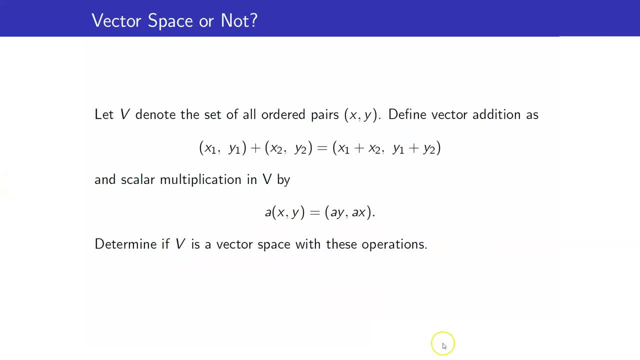 Let's take a look at another example. Again, my set v is a set of all ordered pairs. x, y, x and y are any real numbers. This is our usual addition of ordered pairs, But take note that our scalar multiplication is a bit different. xy. 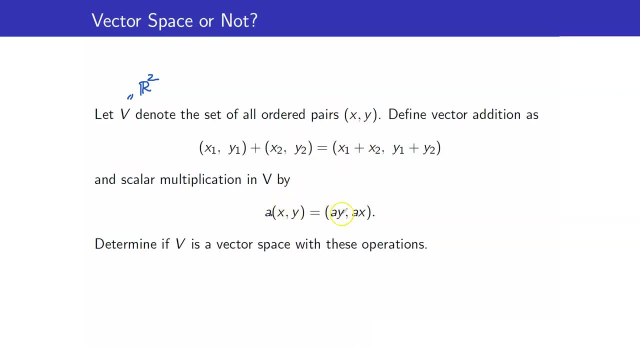 What this does is that it interchanges the two entries. Is v a vector space with this operation, Just like in the previous example. since the scalar multiplication here is a bit different, I would be checking for the axioms concerning scalar multiplication. I will start with the property earlier wherein we have 1.v. 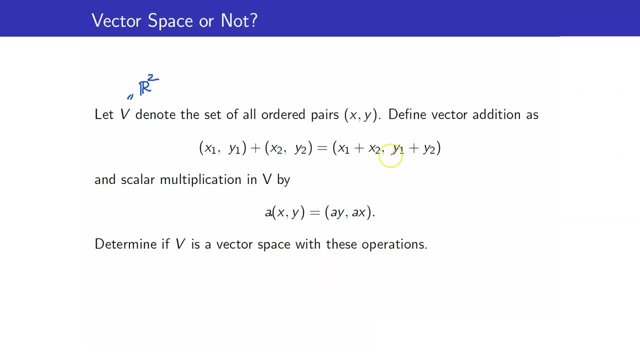 Is that the same as v? Take note that v is closed under addition in scalar multiplication Because this product is again in R2.. This is again in R2.. Therefore it is closed under vector addition in scalar multiplication, Since the scalar multiplication here is a bit different. 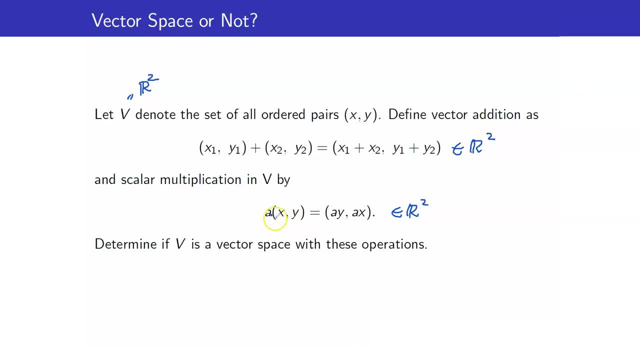 I would start by checking the axioms concerning scalar multiplication. Let me first start with this one. this property 1.v. Is it equal to v? My scalar is 1 times my vector is an ordered pair. Is that equal to xy? 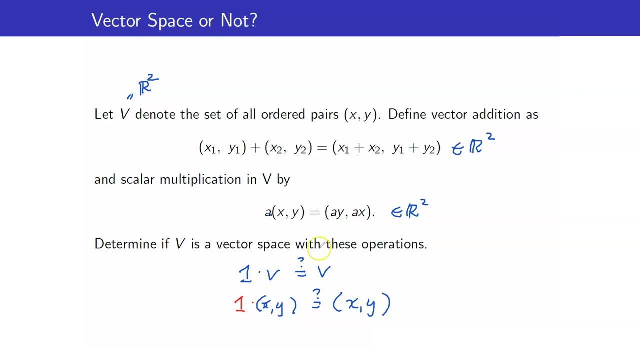 1.xy would be equal. to take note that it will be reversed: It will be 1 times y, 1 times x, And that would not be equal to xy. Therefore, the answer here is no. It suffices to show that one property was not satisfied.